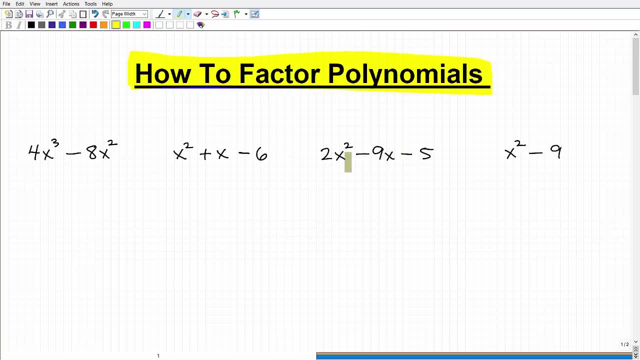 then you're, then you're going to really struggle factoring polynomials. I'll say additionally: if you can't factor polynomials, then you're going to struggle. It's probably going to be impossible for you to pass your algebra class or whatever other math class you might be doing if it involves algebra. So this is an absolutely necessary topic to to learn in math. Okay, so I got four different situations here And let's get into it And if you understand this, you're going to be able to do it. 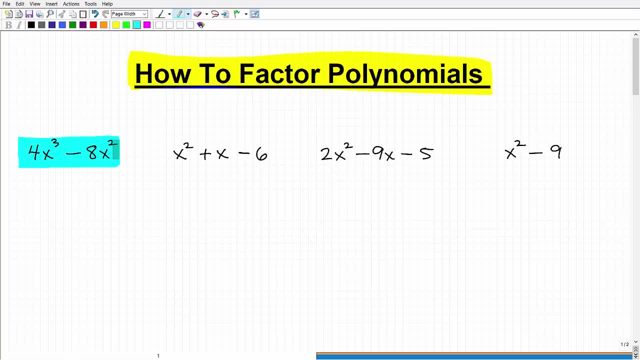 these four scenarios, then you're going to be able to really handle most polynomial factoring problems that you encounter in algebra. All right, so the first is this problem, and this represents the GCF technique. Now, the GCF is the greatest common factor. You always, always, start when 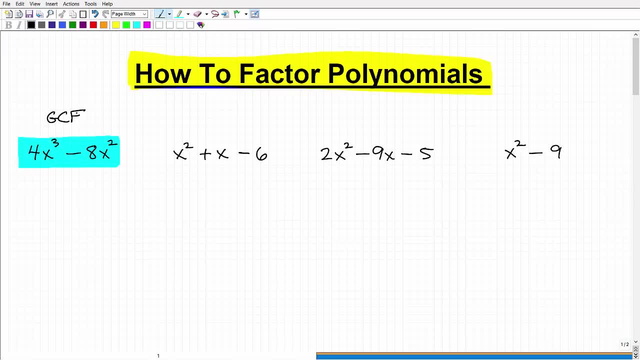 you're looking at a polynomial to see if you can factor out a greatest common factor. Okay, now here you can. So each one of these problems that I have down here are factorable. So if you want to pause the video and just factor them real quick, then that you know. then see my answers. That's. 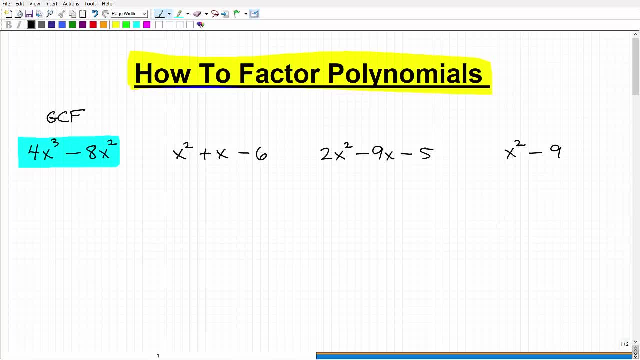 kind of a good little pop quiz for you, And these are pretty simple problems, so I wouldn't get necessarily too overly confident if you can handle these, but that's a good indication that you know what you're doing. But anyways, let's get into this. The greatest common factor is the first. 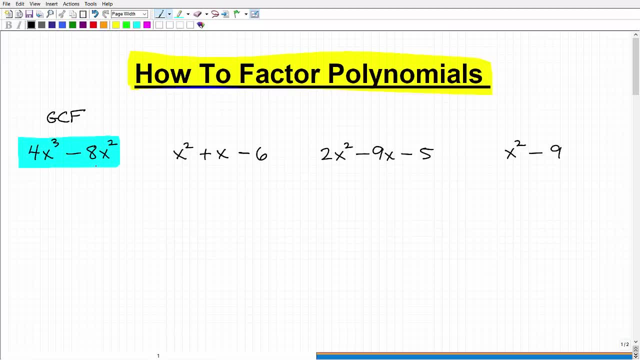 place you always start when you see a polynomial. If you could factor out a greatest common factor, Now here, what that is is the greatest. well, it's exactly what the name says: It's the greatest common factor. So what's common amongst these two? 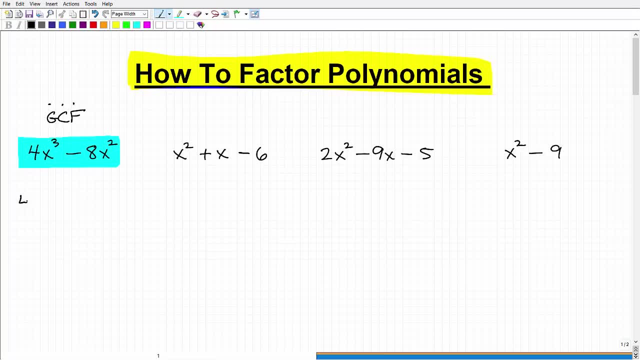 terms here, in terms of a number, Well, it's four, Okay, and then they have the highest power of x. This is x cubed, This is x squared, but they only share an x squared. There is in common, So you would factor out. 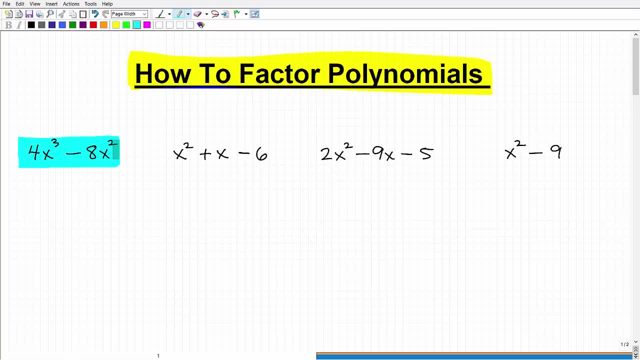 these four scenarios, then you're going to be able to really handle most polynomial factoring problems that you encounter in algebra. All right, so the first is this problem, and this represents the GCF technique. Now, the GCF is the greatest common factor. You always, always, start when 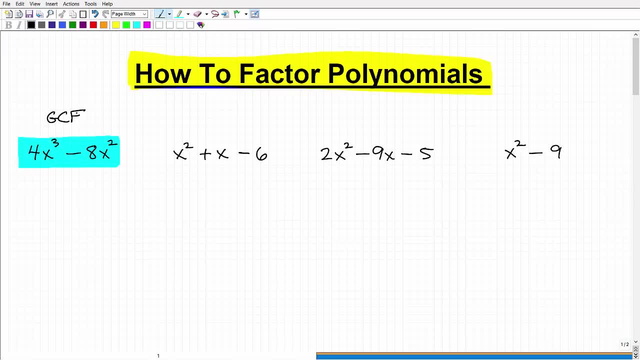 you're looking at a polynomial to see if you can factor out a greatest common factor. Okay, now here you can. So each one of these problems that I have down here are factorable. So if you want to pause the video and just factor them real quick, then that you know. then see my answers. That's. 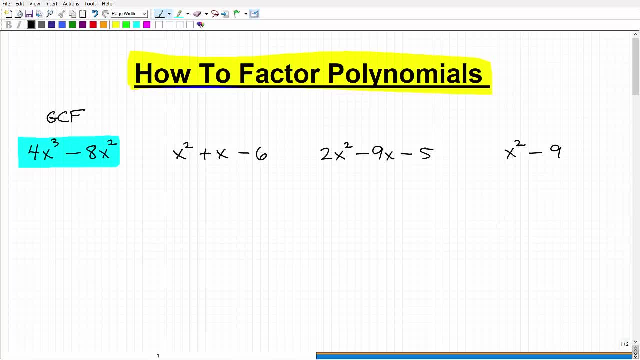 kind of a good little pop quiz for you, And these are pretty simple problems, so I wouldn't get necessarily too overly confident if you can handle these, but that's a good indication that you know what you're doing. But anyways, let's get into this. The greatest common factor is the first. 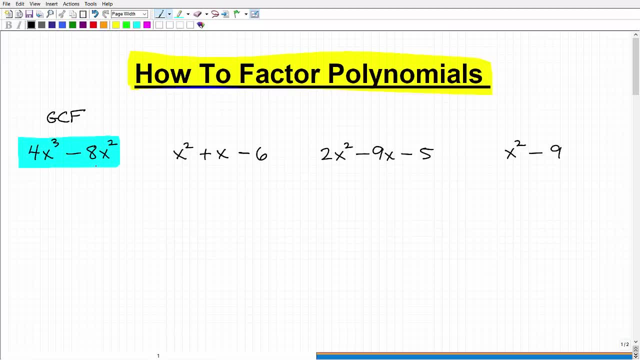 place you always start when you see a polynomial. If you could factor out a greatest common factor, Now here, what that is is the greatest. well, it's exactly what the name says: It's the greatest common factor. So what's common amongst these two? 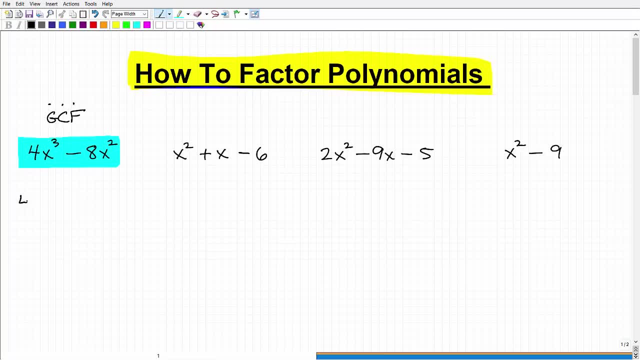 terms here, in terms of a number, Well, it's four, Okay, and then they have the highest power of x. This is x cubed, This is x squared, but they only share an x squared. There is in common, So you would factor out. 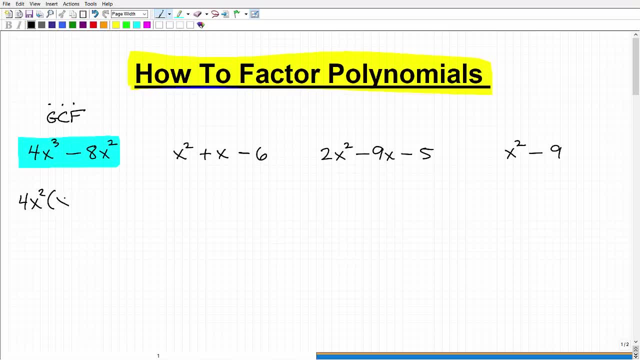 An x squared like so, and that would leave you with an x right here minus two. Okay, Now, if you weren't sure if this was the correct answer, you can multiply these together and you can see you'd get back to this answer. Okay, So this right here for x squared is the greatest common factor. Okay. 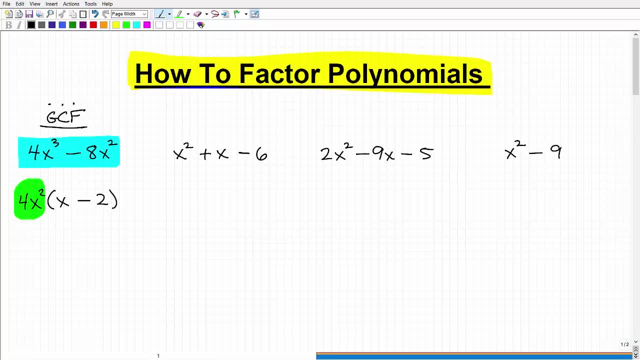 That is the greatest common factor. Now, again, in a short period of time, I'm not going to be able to teach you everything you need to know about the greatest common factor, So you should be somewhat familiar with how to do this. But when it comes to factoring polynomials, this is the number one. 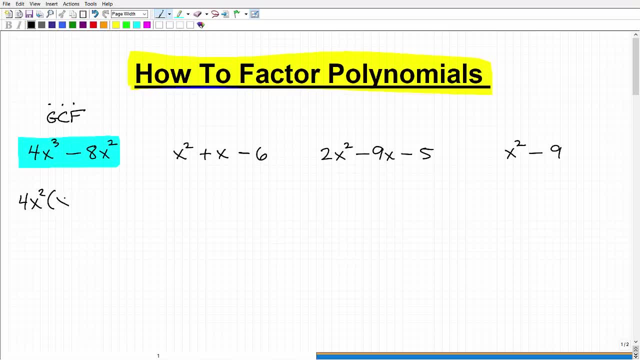 An x squared like so, and that would leave you with an x right here minus two. Okay, Now, if you weren't sure if this was the correct answer, you can multiply these together and you can see you'd get back to this answer. Okay, So this right here for x squared is the greatest common factor. Okay. 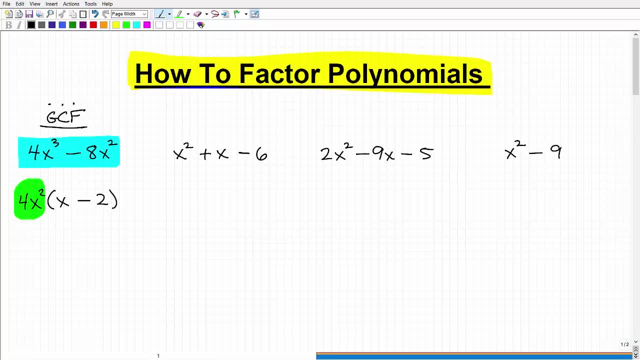 That is the greatest common factor. Now, again, in a short period of time, I'm not going to be able to teach you everything you need to know about the greatest common factor, So you should be somewhat familiar with how to do this. But when it comes to factoring polynomials, this is the number one. 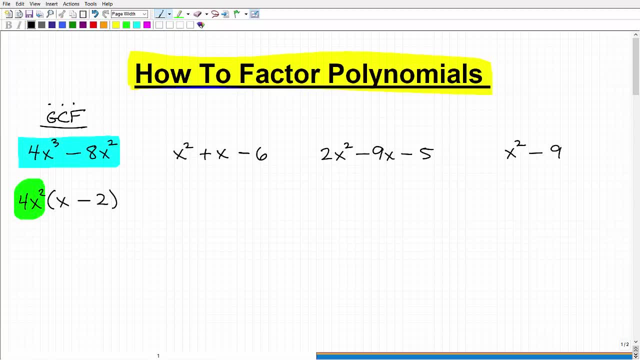 place you want to start. Okay, So if you don't know how to, if you're not comfortable with factoring out the greatest common factor, I have videos on my YouTube channel. I go into it. Plus. you know you might need more extensive instruction, So you might want to check. 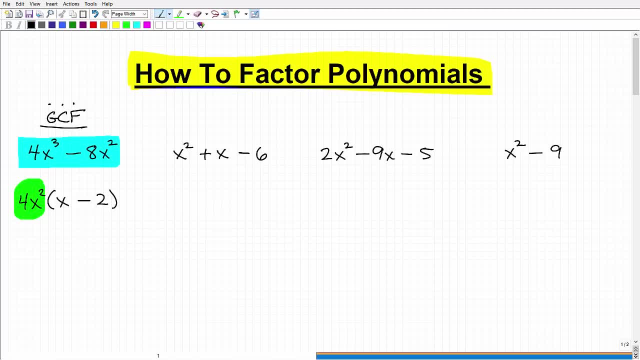 out one of my courses. Just check out the link below. Okay, So that's the first scenario. Okay, Now the second scenario is this: If you can't factor out a greatest common factor, Okay, Let's say you're looking at a polynomial and there is no greatest common factor. Well, that doesn't mean. 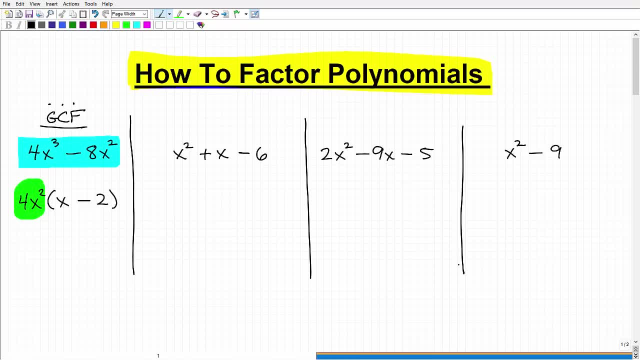 that you're done. Okay. What you may have is one of these three remaining situations, Okay, So let's just kind of talk about these here. So this is what we call a trinomial: There's three terms, but there's no greatest common factor. This is also a trinomial: There's three terms, but there's. 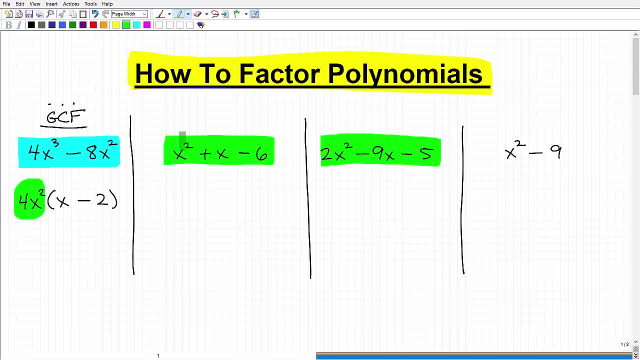 no greatest common factor And the difference between these two trinomials is this: one is just a one x squared, There's just a one in front of it, And then this has a number other than one. So here, in this example, this is two. Okay, So what we have here are trinomials, Trinomials, So this: 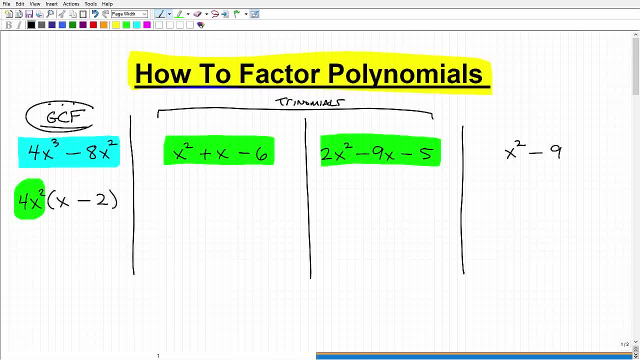 is where you want to look for next. Okay, So you checked out greatest common factors and you're going to see if there's any trinomials. Now the last problem here you might encounter is a special factoring scenario. Okay, So just we'll put the word here. 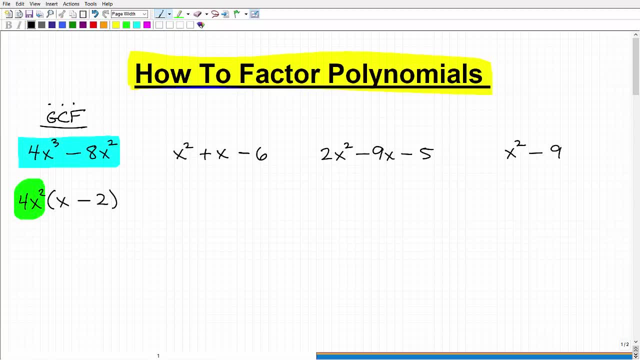 place you want to start. Okay, So if you don't know how to, if you're not comfortable with factoring out the greatest common factor, I have videos on my YouTube channel. I go into it. Plus. you know you might need more extensive instruction, So you might want to check. 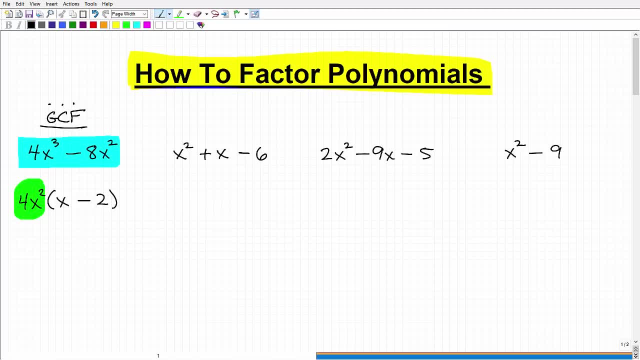 out one of my courses. Just check out the link below. Okay, So that's the first scenario. Okay, Now the second scenario is this: If you can't factor out a greatest common factor, Okay, Let's say you're looking at a polynomial and there is no greatest common factor. Well, that doesn't mean. 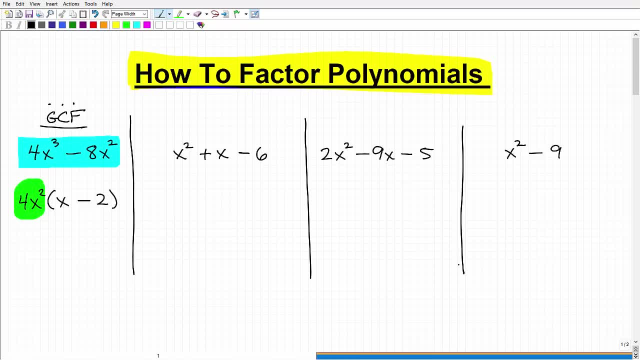 that you're done. Okay. What you may have is one of these three remaining situations, Okay, So let's just kind of talk about these here. So this is what we call a trinomial: There's three terms, but there's no greatest common factor. This is also a trinomial: There's three terms, but there's. 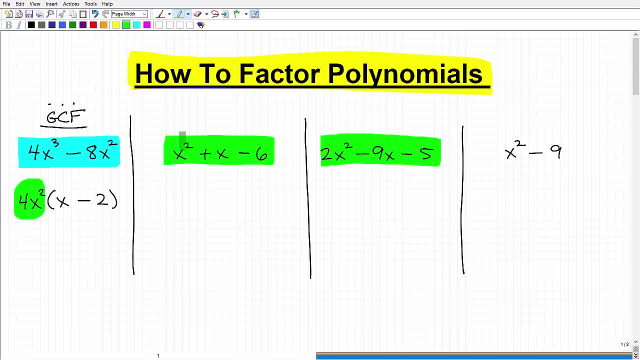 no greatest common factor And the difference between these two trinomials is this: one is just a one x squared, There's just a one in front of it, And then this has a number other than one. So here, in this example, this is two. Okay, So what we have here are trinomials, Trinomials, So this: 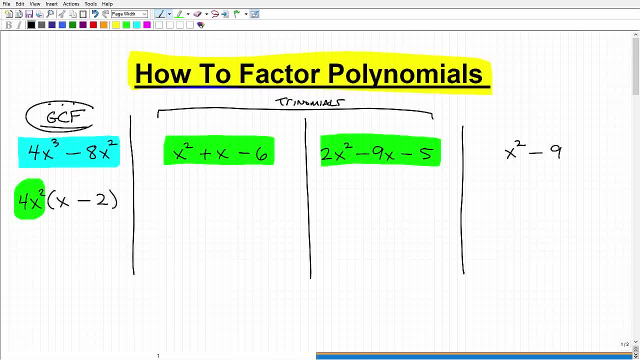 is where you want to look for next. Okay, So you checked out greatest common factors and you're going to see if there's any trinomials. Now the last problem here you might encounter is a special factoring scenario. Okay, So just we'll put the word here. 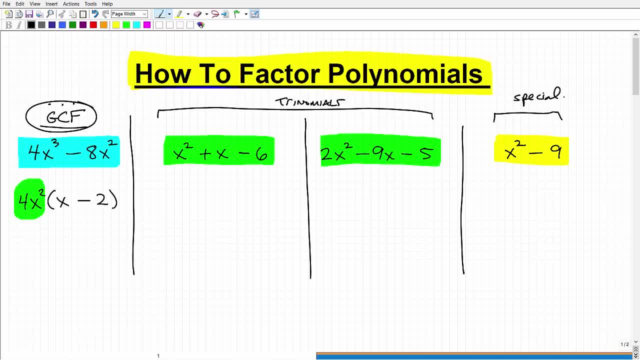 special. So these four scenarios here, four situations, will cover the majority of your factoring scenarios. Okay, Now I'm going to get into these problems, these last three problems here in a second, but I just wanted to just lay out the kind of like your mental organization in terms of: hey, I got to factor a polynomial. 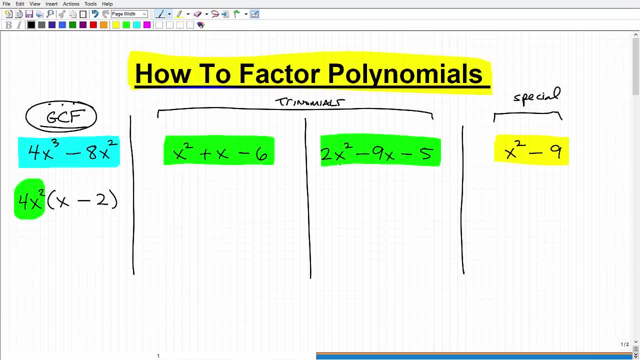 let me start with the GCF. If I'm dealing with a trinomial, what type is it? I like to refer to this as a case one, because there's a one in front of it, And then anything else is what we call like. 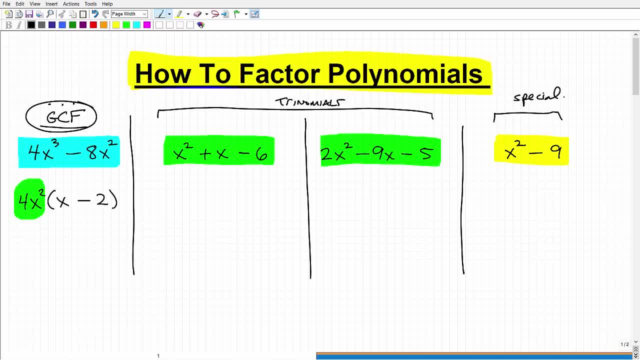 special. So these four scenarios here, four situations, will cover the majority of your factoring scenarios. Okay, Now I'm going to get into these problems, these last three problems here in a second, but I just wanted to just lay out the kind of like your mental organization in terms of: hey, I got to factor a polynomial. 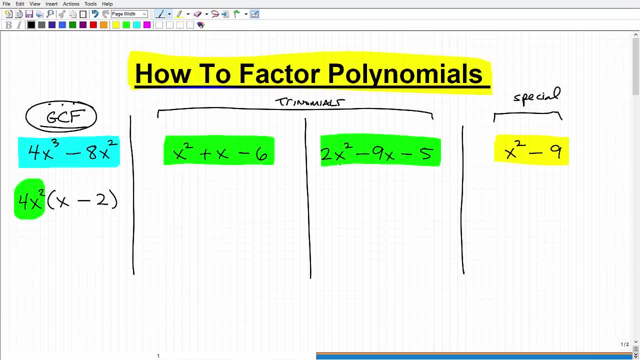 let me start with the GCF. If I'm dealing with a trinomial, what type is it? I like to refer to this as a case one, because there's a one in front of it, And then anything else is what we call like. 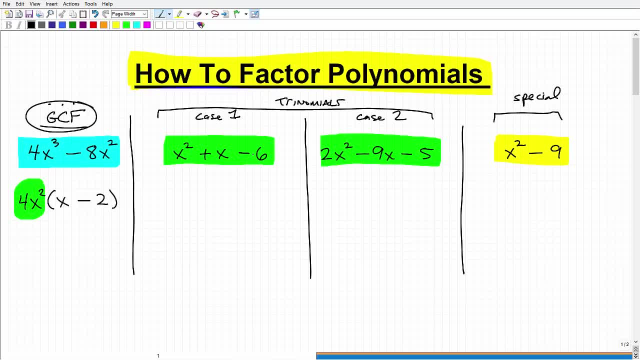 say a case two, All right, And if you don't have a case one or case two, then see if there's any special factoring rules that could apply to the polynomial. Okay, So let's get into this. So very briefly, a case one is a trinomial. 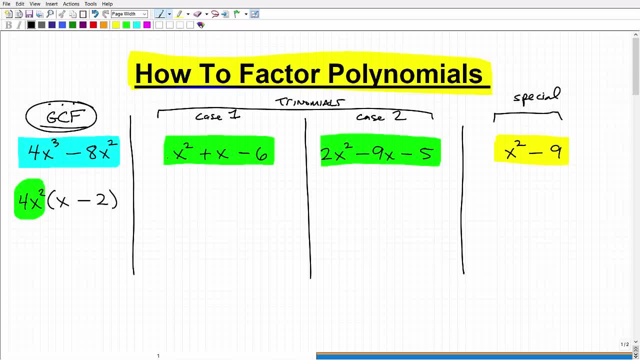 where there's just a one in front of the leading. the one is the leading coefficient. Okay, So when you write it in standard form, So if you look here, the easiest way to factor a case one- if they are factorable- okay, let me just do it this way- is look at this last number. Okay, 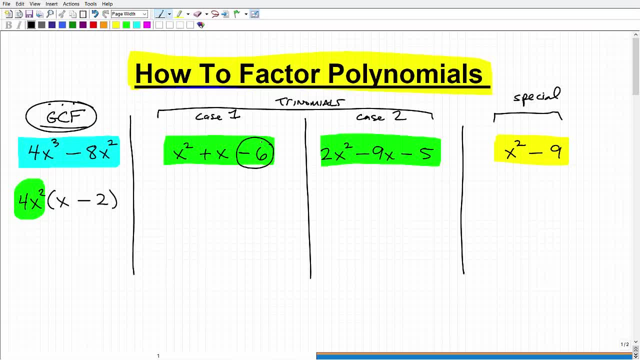 That's negative six. Now one way I kind of like to start students off a factor in case ones is to write out all the factors that are factorable. So let's say I have a case one and I have a case two. 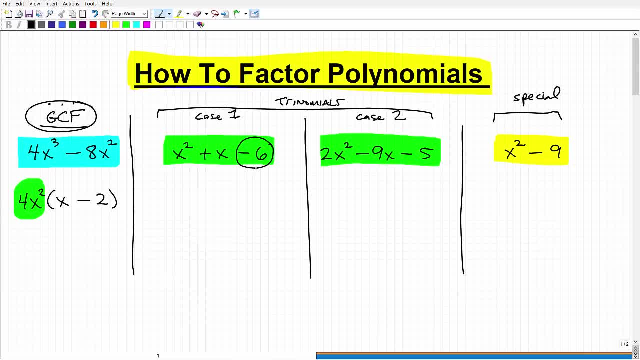 all the factors of a negative six. So here's how you do. Okay, So negative six. you can write as one times six a negative one times six. right, We'll give you a negative six. One times a negative six will give you a negative six. Okay, Two times three, negative, two times three and two times. 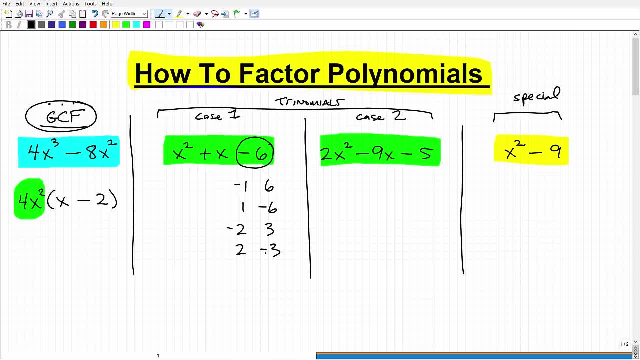 negative three. So these are all the different ways you can write the factors of negative six, right? These different combinations, when you multiply these pairs together, will get you a negative six. Now, if you add up each one of these pairs, which, what do you get? here You get a positive five. 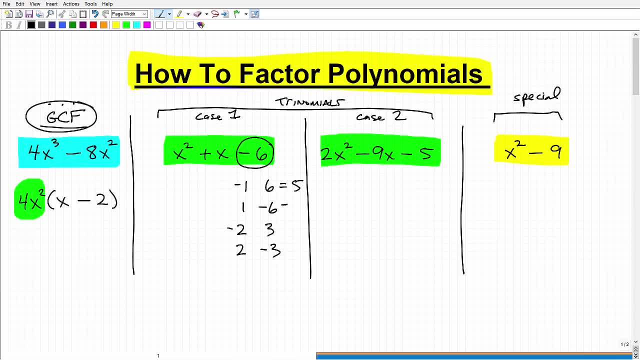 right. Negative. one plus six is a positive five. One plus negative six is negative five. This right, here is a one and this is a negative one, right? So when you add all these pairs together, So what you want to do is to see if you have a pair, any pairs of factors that 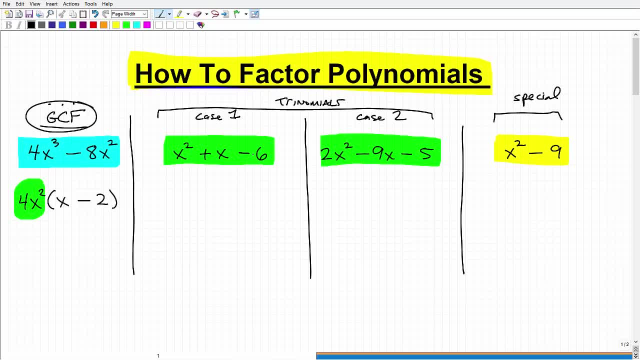 say a case two, All right, And if you don't have a case one or case two, then see if there's any special factoring rules that could apply to the polynomial. Okay, So let's get into this. So very briefly, a case one is a trinomial. 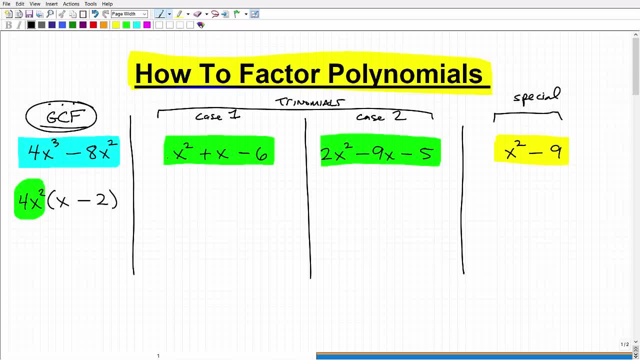 where there's just a one in front of the leading. the one is the leading coefficient. Okay, So when you write it in standard form, So if you look here, the easiest way to factor a case one- if they are factorable- okay, let me just do it this way- is look at this last number. Okay, 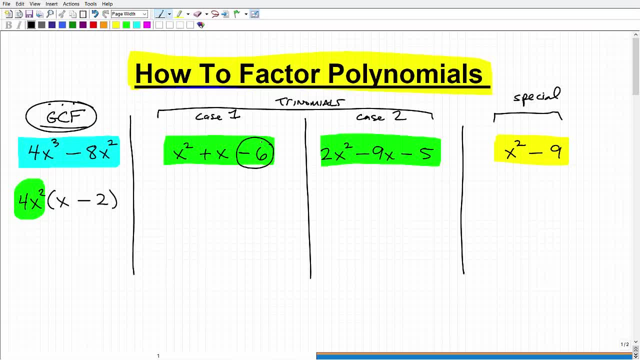 That's negative six. Now one way I kind of like to start students off a factor in case ones is to write out all the factors that are factorable. So let's say I have a case one and I have a case two. 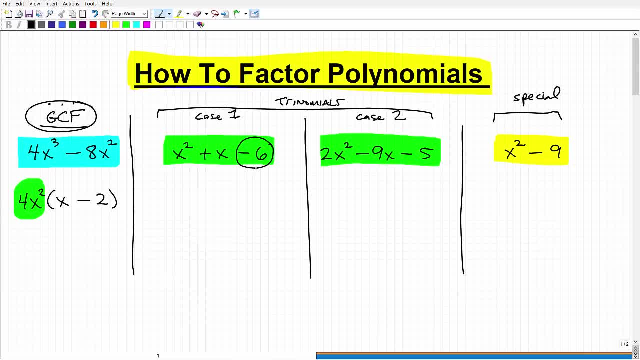 all the factors of a negative six. So here's how you do. Okay, So negative six. you can write as one times six a negative one times six. right, We'll give you a negative six. One times a negative six will give you a negative six. Okay, Two times three, negative, two times three and two times. 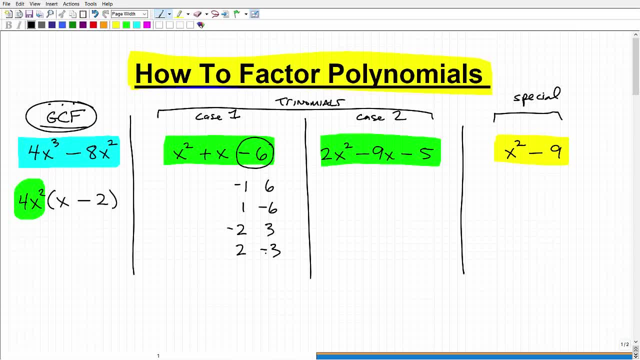 negative three. So these are all the different ways you can write the factors of negative six, right? So if you add up all these numbers, these different combinations, when you multiply these pairs together, we'll get you a negative six. Now, if you add up each one of these pairs, which, what do? 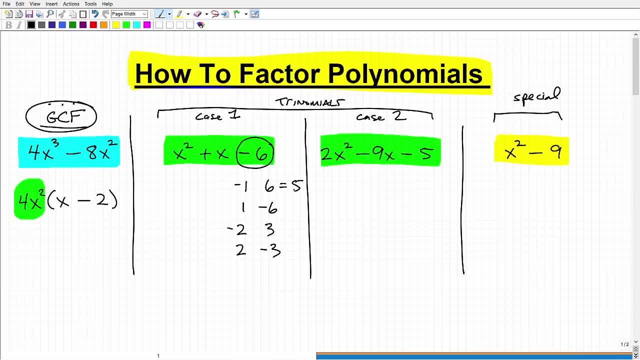 you get here, You get a positive five, right. Negative one plus six is a positive five. One plus negative six is negative five. This right here is a one and this is a negative one, right? So when you add all these pairs together. So what you want to do is to see if you have a pair. 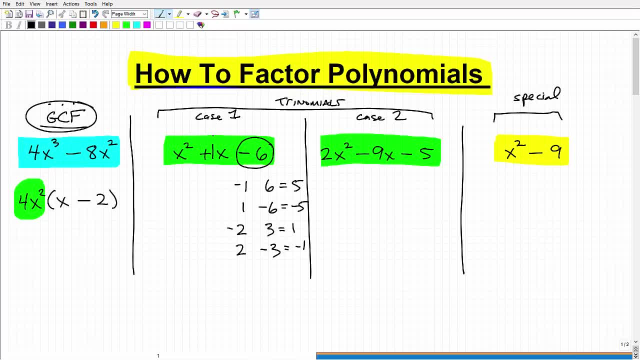 any pairs of factors that add up and you get a positive five, you get a negative five And that's going to add up to this center number. okay, So this is a one x squared, This is a positive one. So which one of these pairs adds up to a positive one? It's these pairs, right? Negative two plus. 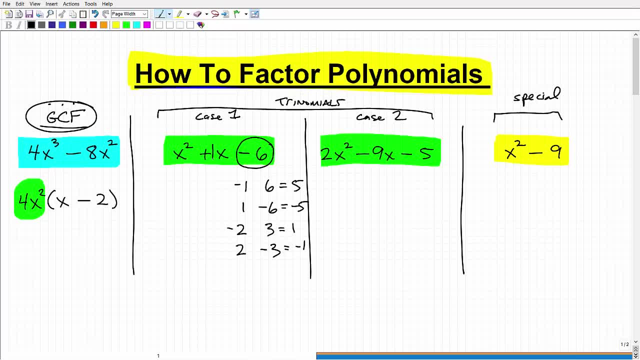 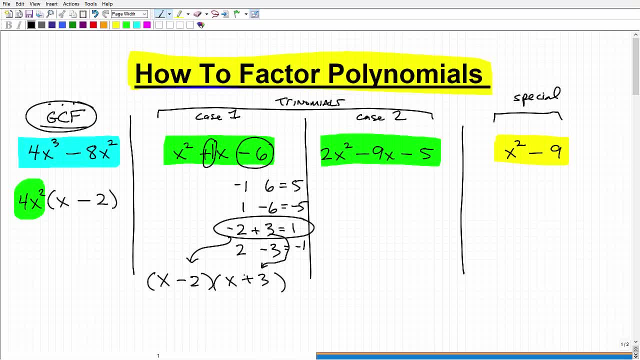 plus three right there. so these are the factors to that trinomial. it's as simple as that. okay, of course, you need to practice this now. if you couldn't find any pairs of factors here that add up to that center number, then a factor and then the polynomial is unfactable. it's what we call prime. okay, so let's move on. 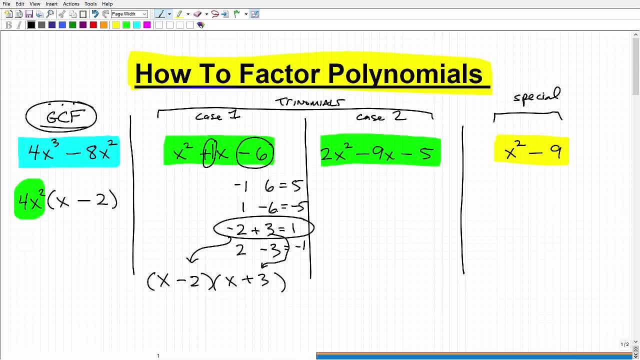 to this case two. now the case two: you could do, you can do this in a similar manner, but there's some additional steps. but I'm gonna give you another technique you can use to try to factor a case. to let me write this a little better. I kind of call it the double smiley face. so the first thing is we 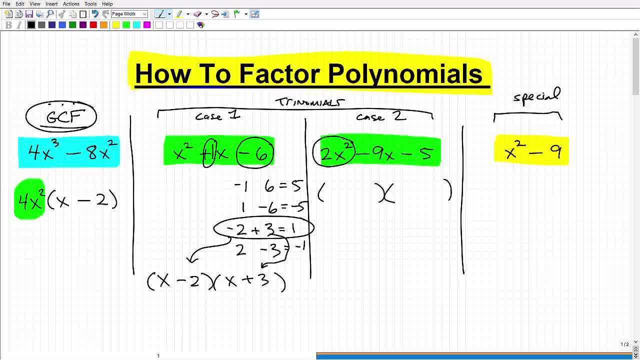 have 2x squared. so you want to write the factors of 2x squared, doesn't? there's only one way to factor that, and that would be a 2x and X, right? so if I multiply 2x and X together, I get a 2x squared. there's no other way I could. 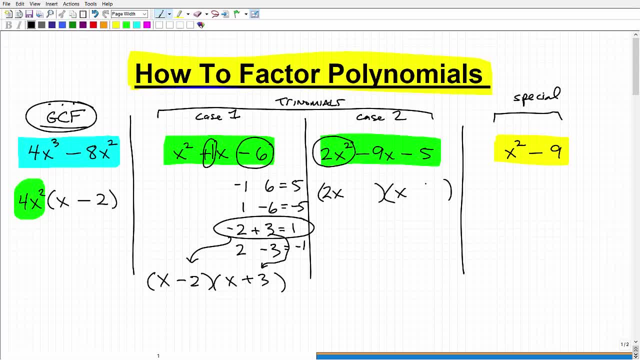 write that now. what we're trying to do here is play a little game to try to get back to this center number now the way we have to do that is write the factors of negative 5 in this position right here. you'll see how this comes together here in a second. 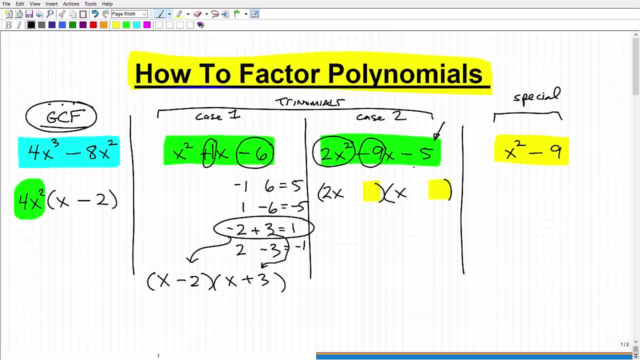 so negative 5 is what? 1 times negative 5, or negative 5 times 1? so I'm gonna put this negative 5 right there and I'm gonna put a 1 right there. okay now, if, what, if what? what I'm going to show you doesn't work. I can just kind of maneuver these combinations around. 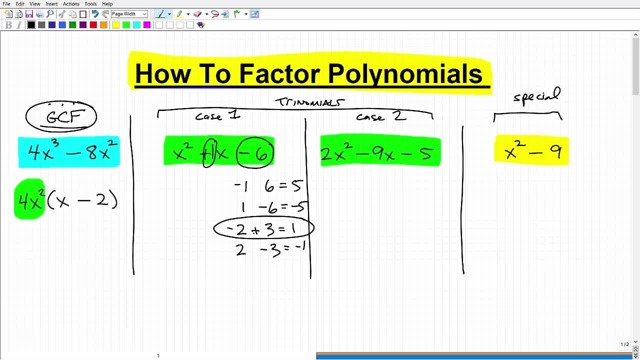 three gives you a positive one. And these are the answers, These are the factors. So you could write this trinomial, you can factor it this way: Okay, You're always going to have two binomials, So it's going to be x minus two. okay, One of those answers And x minus two. 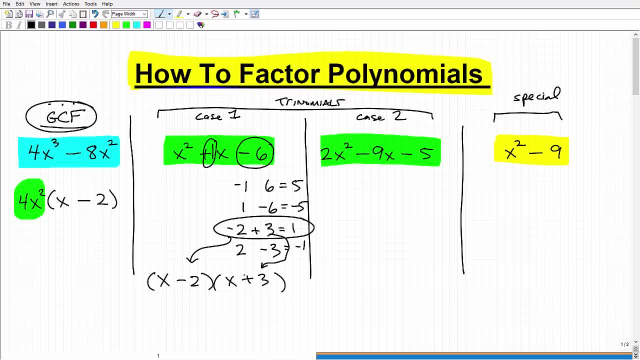 x plus three. right there. So these are the factors to that trinomial. It's as simple as that. okay, Of course, you need to practice this Now. if you couldn't find any pairs of factors here that add up to that center number, then the polynomial is unfactable. It's what we call prime. 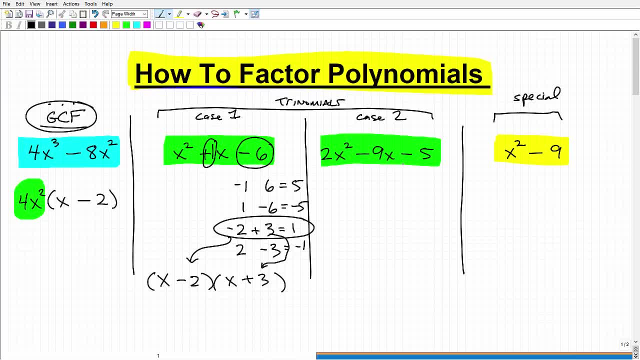 okay, So let's move on to this case two. Now the case two. you can do this in a similar manner, but there's some additional steps. but I'm going to give you another technique you can use to try to factor a case two. Let me. 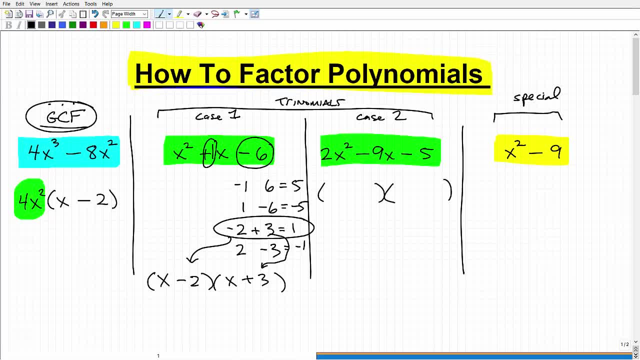 write this a little better. I kind of call it the double smiley face. So the first thing is we have two x squared, So you want to write the factors of two x squared. There's only one way to factor that, and that would be a two x and an x, right? So if I multiply two x and x together, 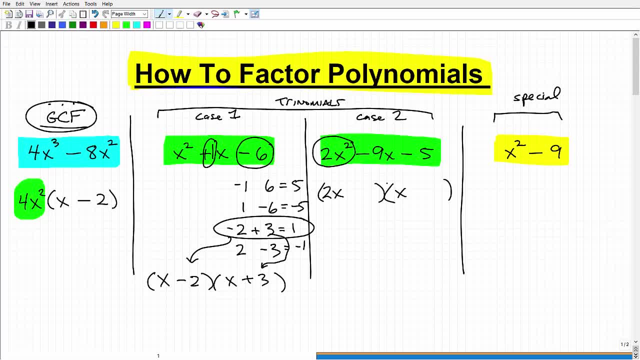 I get a two x squared. There's no other way I could write that. Now, what we're trying to do here is play a little game to try to get back to this center number. Now, the way we have to do that is write the factors of negative five in this position right here. You'll see how this comes. 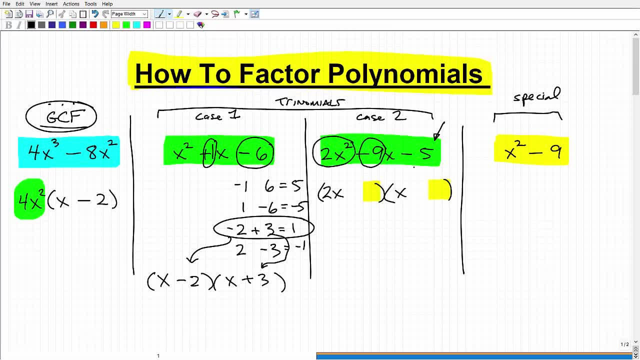 together here in a second. So negative five is what? One times negative five, or negative five times one? So I'm going to put this negative five right there and I'm going to put a one right there. okay, Now, if what I'm going to show you doesn't work, I can just give you a little bit of 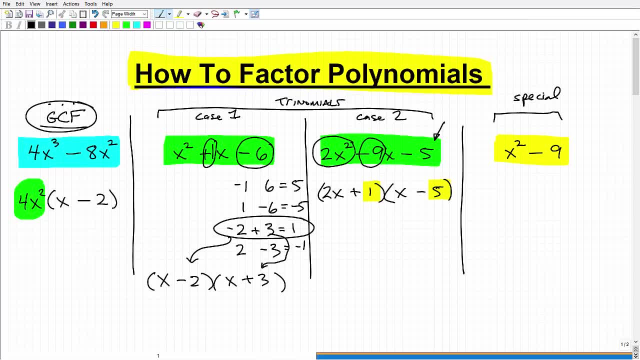 kind of maneuver these combinations around, because I'm trying to get back to the center number Now. I told you I was going to use something called the double smiley face technique. So what that is is: you take this number here and you multiply it by this, okay, And that's one smiley face. 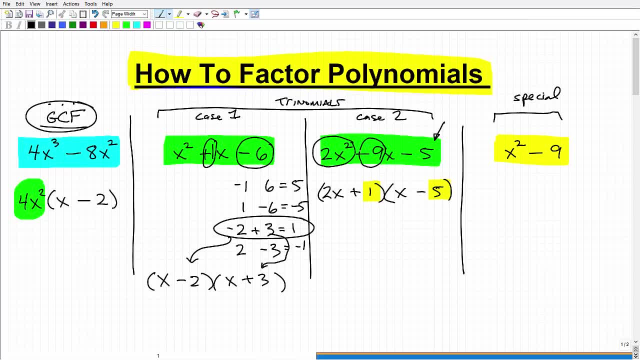 because I'm trying to get back to the center number Now. I told you I was going to use something called the double smiley face technique. So what that is is you take this number here and you multiply it by this, okay, and that's one smiley face, if you will. and then we do this. 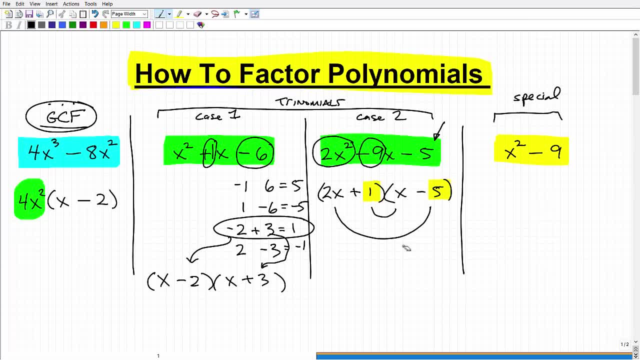 times this. So you can see we have two smiley faces. Let me draw this other one a little bit bigger. Okay, so we have 1x, right. 1 times x is x, or 1 times x is 1x, positive 1x. 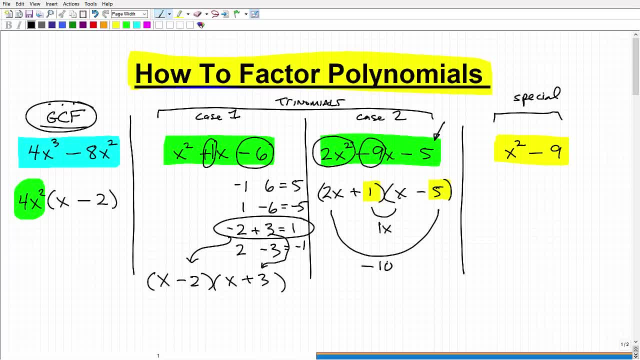 and then I have 2x times a negative 5, that's negative 10x. Now if I add these two guys together, you're looking to see which combination gets back to the center term. So if you see here, 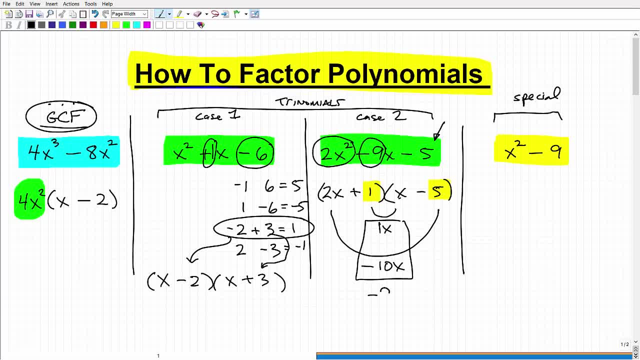 a 1x. a positive 1x plus a negative 10x gets me a negative 9x. So the these factors right here are correct, okay, because of that, and if you wanted to, you can just multiply all this out to verify that, in fact, you have the correct factors, okay, So. 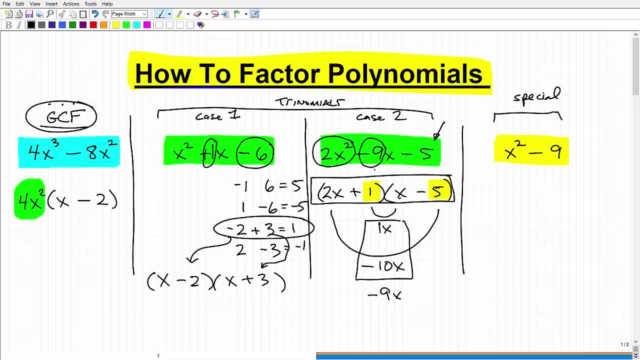 this is the double smiley face. Now you could do this problem in a similar fashion as I did this first case, one problem, but there's some additional steps. So I really like the double smiley face technique. for this case, two polynomials and for case one, this technique I showed you here is: 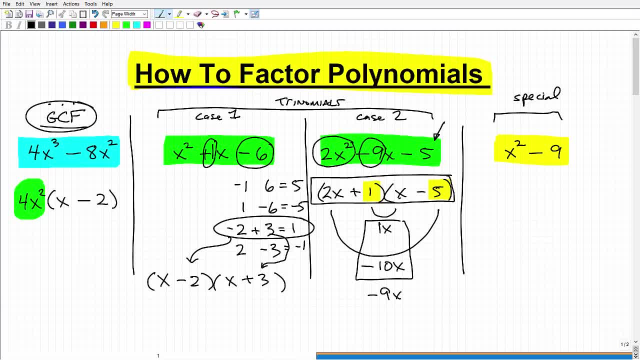 just really straightforward, okay, So I would suggest using that as well. Okay, so now you have three things. we have three things behind us, right? We have the greatest common factor. we always look there first. then, if we're dealing with trinomials, what type? and if we don't have, 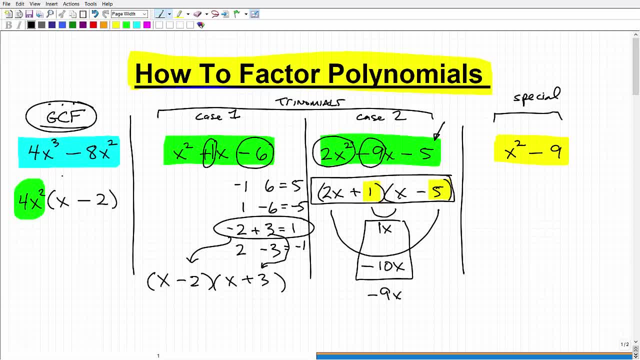 any trinomials. we don't have any greatest common factor. that doesn't mean that you're done. You may have a special factoring scenario. So if you look here, this last problem: there's no GCF, it's not a trinomial. so what do you do? 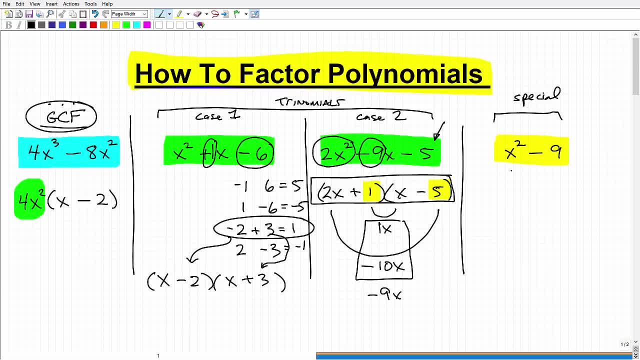 Well, in this case, you just need to know the special factoring rules. Probably one of the most important is a squared minus b squared. let me write this this way here: a squared minus b squared is equal to a plus b, times a minus b, It's called the difference of two squares. It's. 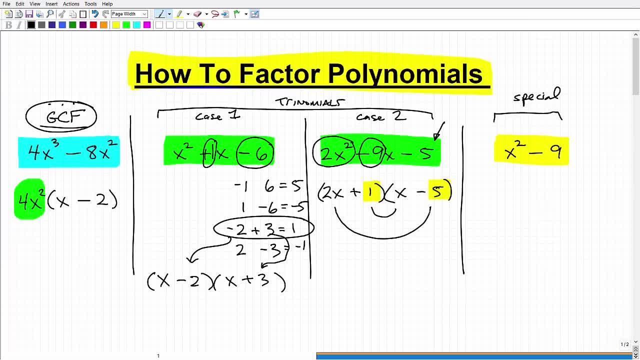 if you will, And then we do this times this, So you can see we have two smiley faces. Let me draw this other one a little bit bigger. Okay, so we have one x, right? One times x is one x, or one times x is one x, positive one x, And then I have two x times a negative five, that's. 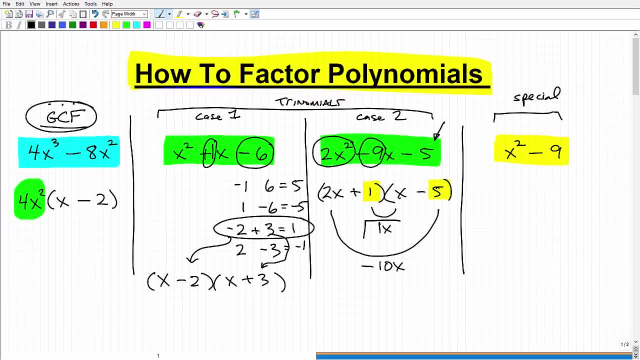 negative 10x. Now if I add these two guys together, you're looking to see which combination gets back to the center term. So if you see here a one x, a positive one x plus a negative 10x gets me a negative nine x. So these factors right here are correct. okay, because of that, And if you 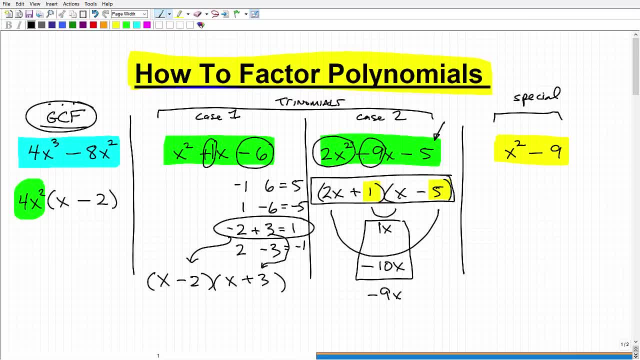 wanted to, you can just multiply them. So if you wanted to, you can just multiply them. So if you want to multiply all this out to verify that in fact you have the correct factors, okay, So this is the double smiley face. Now you could do this problem in a similar fashion as I did this first. 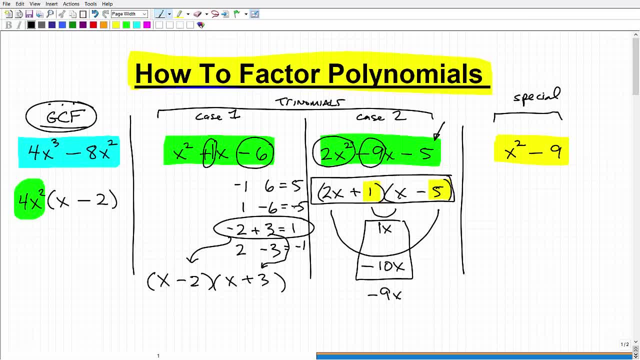 case one problem, but there's some additional steps. So I really like the double smiley face technique for this case, two polynomials And for case one, this technique I showed you here is just really straightforward. okay, So I would suggest using that as well. Okay so. 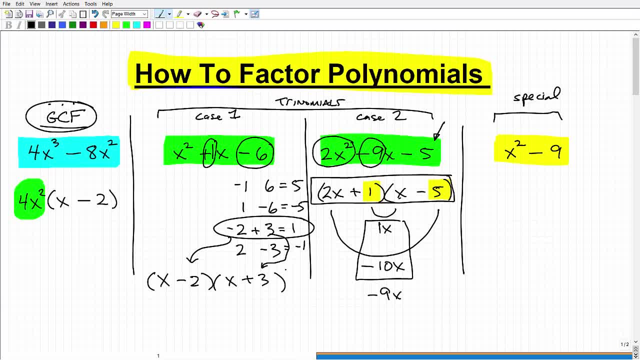 now you have three things. We have three things behind us. right, We have the greatest common factor. We always look there first. Then if we're dealing with trinomials, what type? And if we don't have any trinomials, we don't have any greatest common factor. that doesn't mean that you're done. 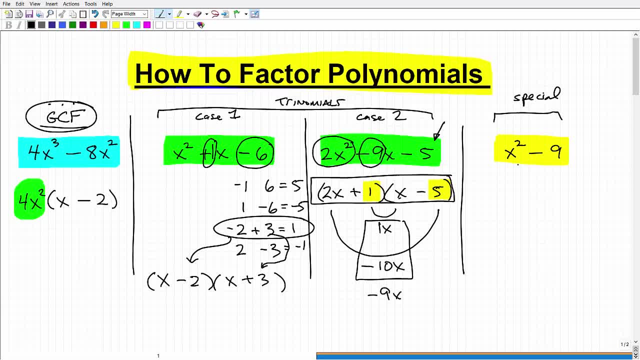 You may have a special factoring scenario. So if you look here, this last problem, there's no GCF, It's not a trinomial. So what do you do? Well, in this case, you just need to know the special factoring rules. Probably one of the most important is a 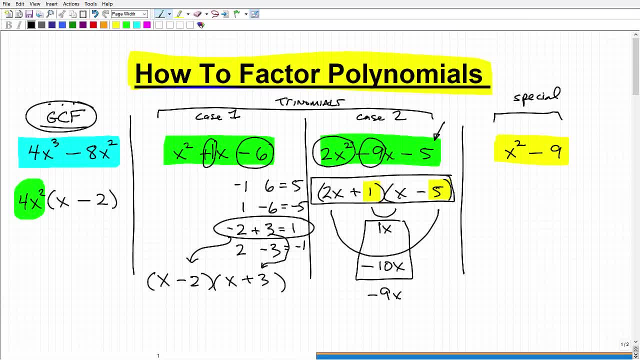 squared minus b squared. Let me write this this way: here, a squared minus b squared is equal to a plus b times a minus b. It's called the difference of two squares. It's used extensively, okay, when we're talking about factoring. So here the way I would factor this. I would just simply: 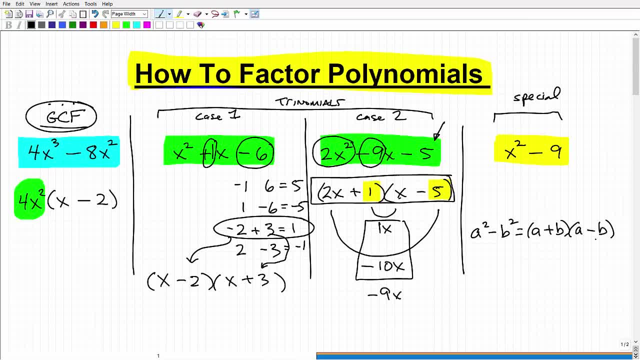 used extensively. okay, when we're talking about factoring. So here the way I would factor this: I would just simply need to know this rule. This is a special factoring rule, So this is going to be x plus three times x minus three. 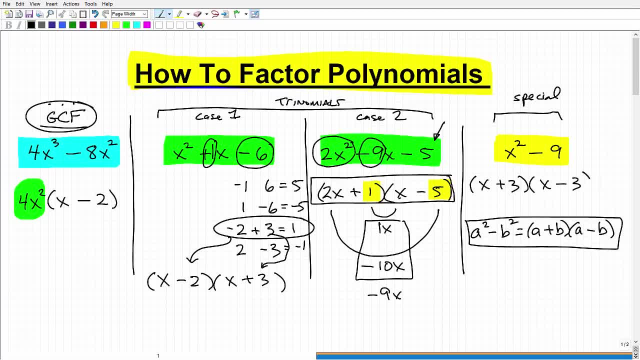 okay, I'll write that a little bit better. So this is how this factors here, because I know the special factoring rule. Now again, I'm going to wrap up this video here. No way could I fit in what takes your teacher a couple weeks to teach you At least the factoring is. 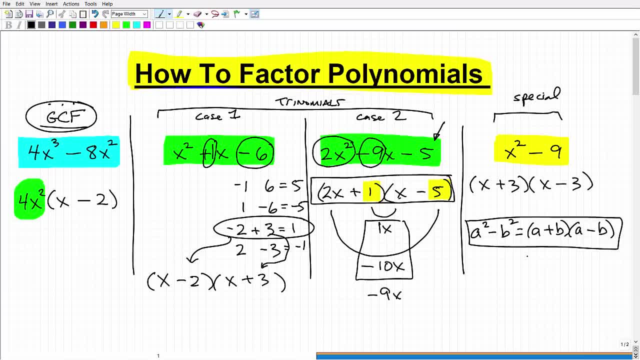 covered in you know in over and over in multiple math courses. So this is a lot of you know skills, that kind of build up. No way should you expect to just watch this video and be like a total expert. but if you have a clue about factoring and you know how to multiply and 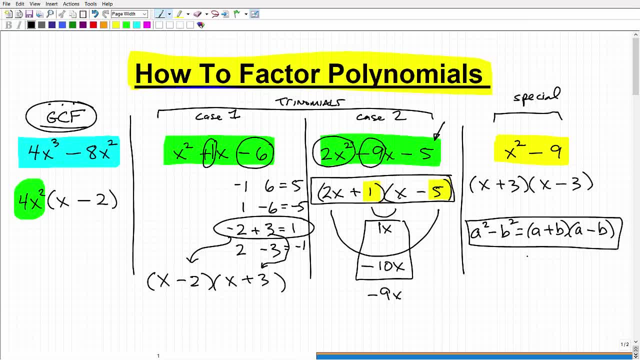 you're like, oh, you're just kind of struggling or a little bit confused, then I think this video would definitely should have helped you out. right, Because you always start here, You'll always start with the GCF. Then look to see if you have any of these scenarios and then, if you, 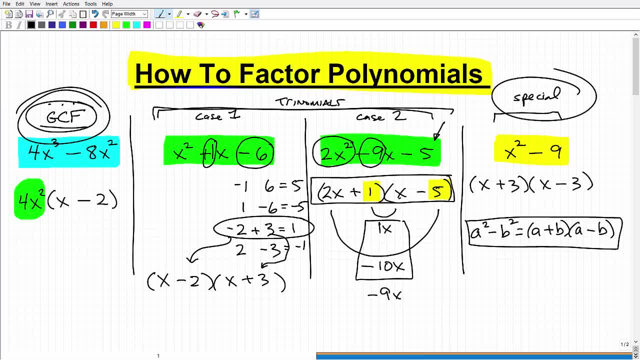 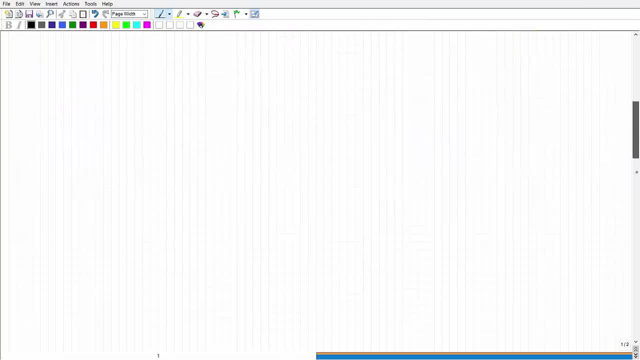 don't just make sure you don't have any special scenarios. If you follow this, you're going to be good to go in most factoring situations. but again, if you need more help, you want to go ahead and check out some additional videos I have on my YouTube channel, So please consider subscribing. 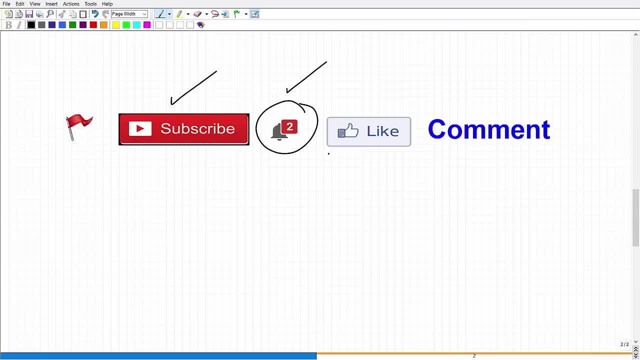 and if you do hit that bell notification and if you like this video- hey, you know, give me a thumbs up- I appreciate that- and leave me comments. It's one of the things that I try to read. I do get a lot of comments on my videos, which I'm grateful for. 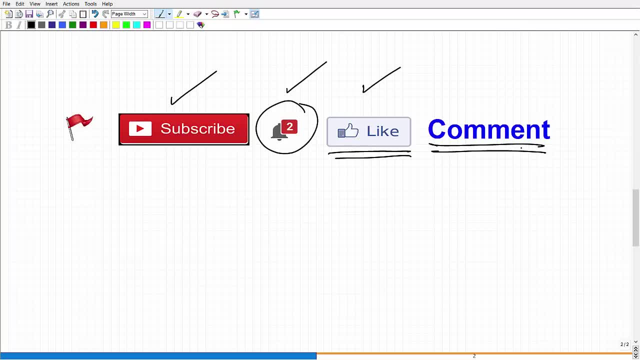 But it gives me feedback on videos- future videos I can make that are going to help you out Again. you know, if you like my teaching style and you understand you know how I teach and you need extensive help in math, then you might want to consider checking out some of my 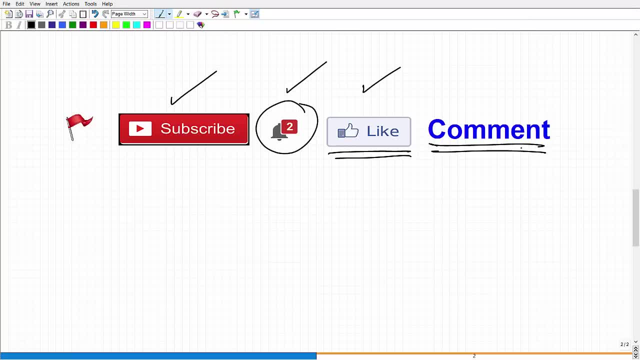 math courses and I'll leave a link in the description in the video if you're interested there. But other than that, I appreciate your time and have a great day. 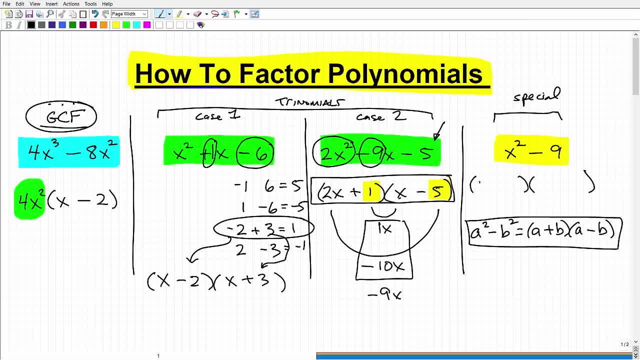 need to know this rule. This is a special factoring rule, So this is going to be x plus 3 times x 3, okay, I'll write that a little bit better. So this is how this factors here, because I know. 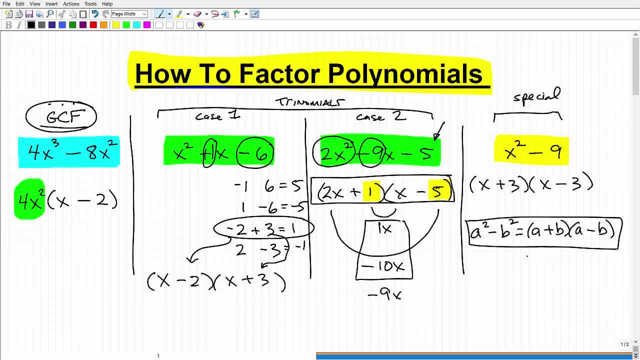 the special factoring rule. Now again, I'm going to wrap up this video here. No way could I fit in what takes your teacher a couple weeks to teach you. At least factoring is covered in, you know, in over and over in multiple math courses. So this is, this is a lot of you know. 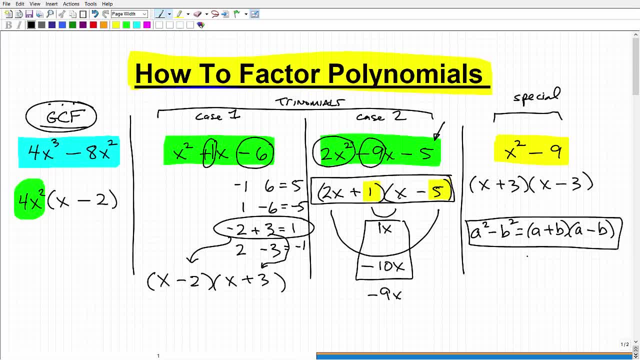 skills, that kind of build up. No way should you expect to just watch this video and be like a total expert. But if you have a clue about factoring and you know how to multiply and you're like, oh, you're just kind of struggling or a little bit confused, then I think this video 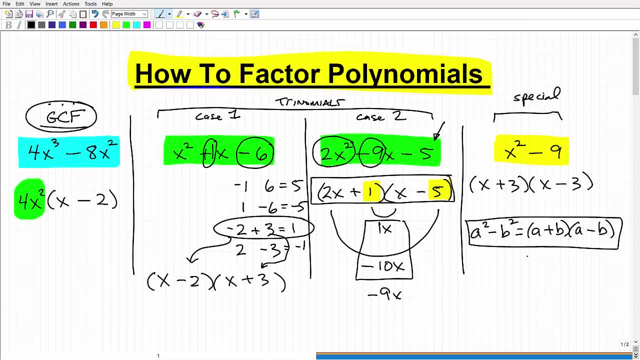 would definitely should have helped you out, right? Because you always start here, You always start with the GCF. Then you look to see if you have any of these scenarios And then if you don't, just make sure you don't have any special scenarios, If you follow this, you're going to be. 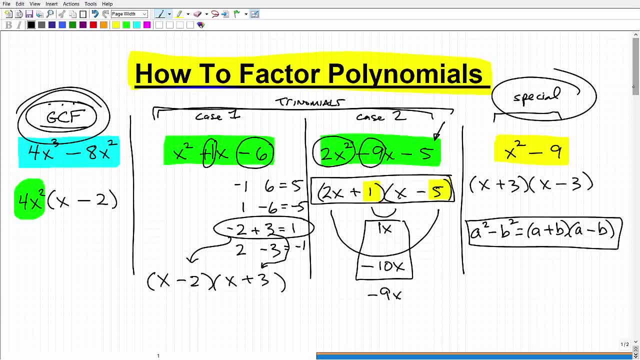 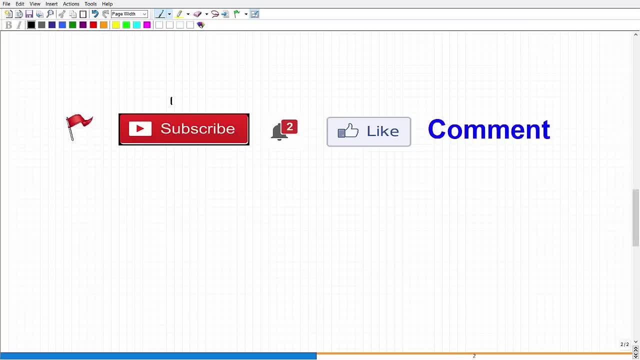 good to go in most factoring situations. But again, if you need more help, you want to go ahead and check out some additional videos I have on my YouTube channel. So please consider subscribing And if you do, hit that bell notification And if you. 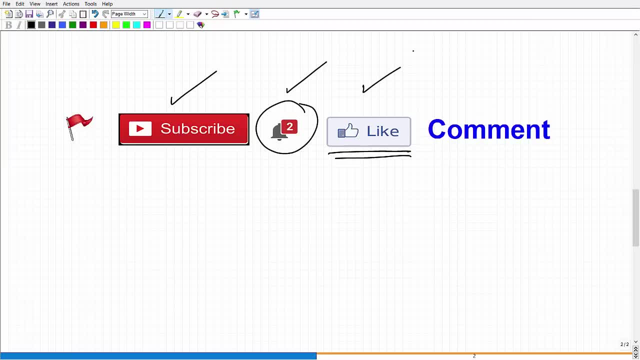 like this video. hey, you know, give me a thumbs up- I appreciate that- And leave me comments. It's one of the things that I try to read it. I do get a lot of comments on my videos, which I'm grateful. 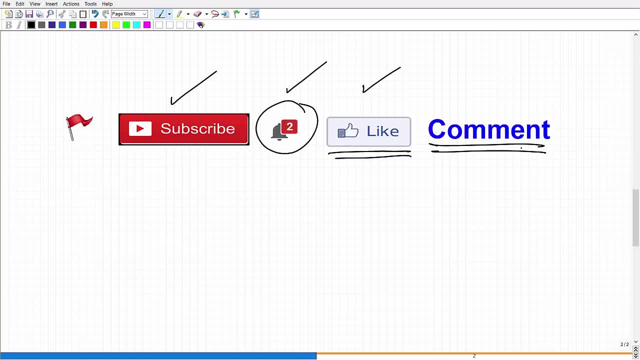 for, But it gives me feedback on on videos that I future videos I can make that are going to help help you out Again. you know, if you like my teachings down, you understand, you know. you know how I teach. 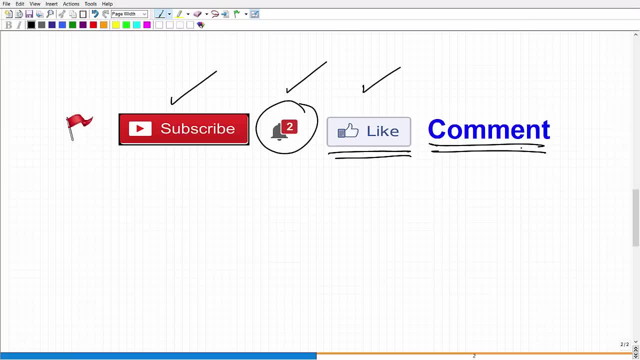 and you need extensive help in math, then you might want to consider checking out some of my math courses And I'll leave a link in the description in the video if you're interested there. But other than that, I appreciate your time and have a great day.